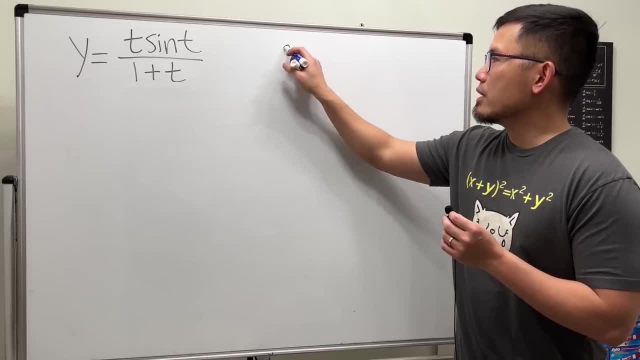 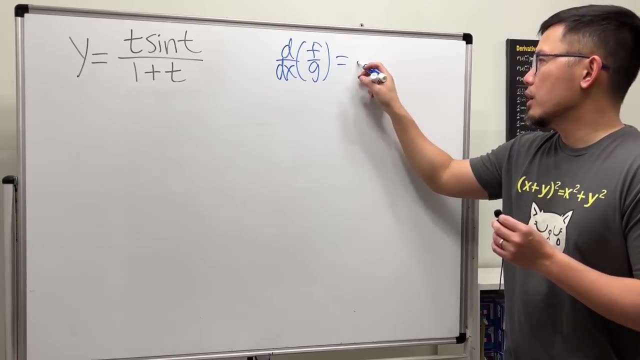 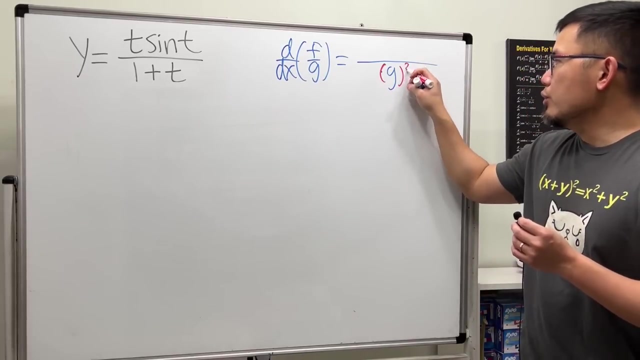 quotient rule. and let me remind you right here, first, Today, if we are trying to differentiate a quotient of two functions, f over g, this right here, let's go ahead and square the denominator first, So g squared, and then for the numerator we write down the bottom function times, the 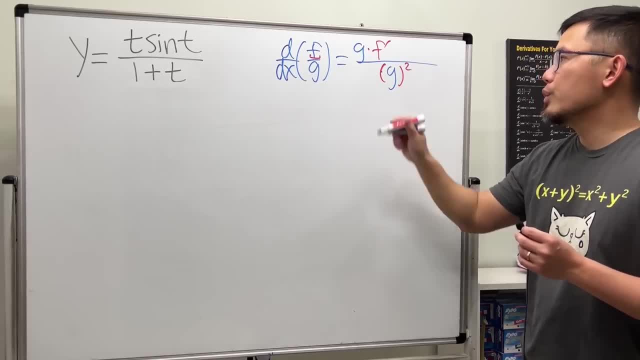 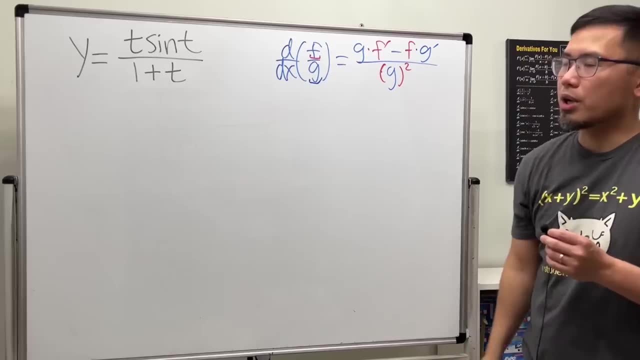 derivative of the first, which is f prime, and then we will have to subtract the top function times, the derivative of the bottom, which is denoted by g prime. So, that said, let's go ahead and see how we can differentiate t times sin t over 1 plus t. So by the look of it, we know that. 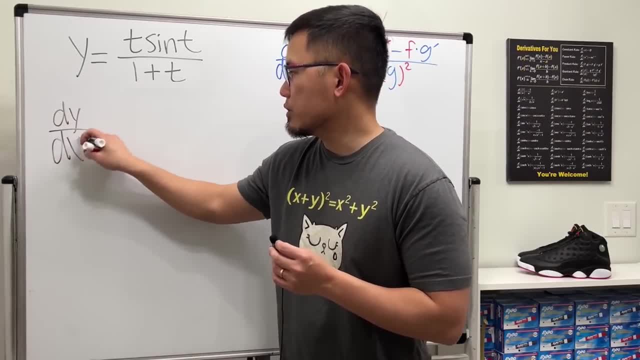 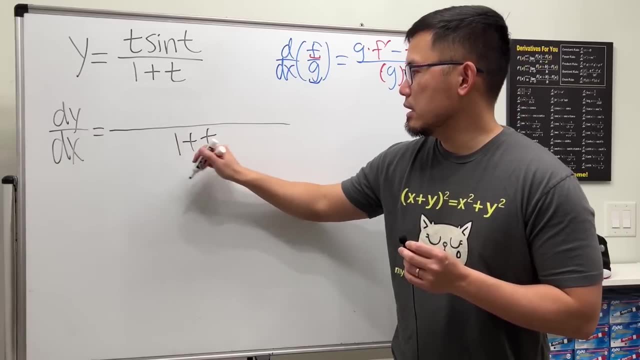 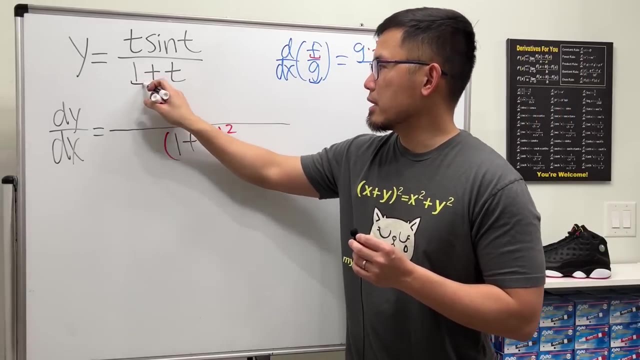 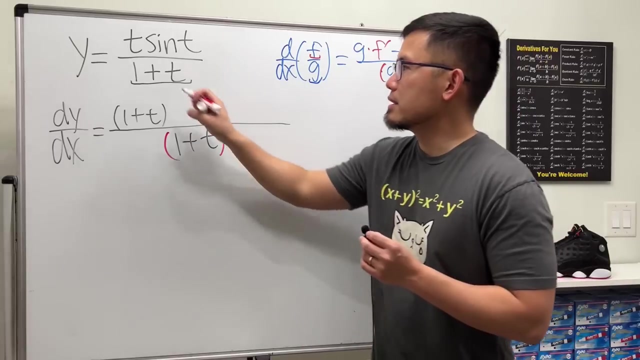 I will use dy, dx for the derivative notation and let's go ahead and square the denominator before we forget. So 1 plus t and then squared. Then I'm going to write down the bottom function right here. This is the bottom function. We have 1 plus t done. Now the trick part is: 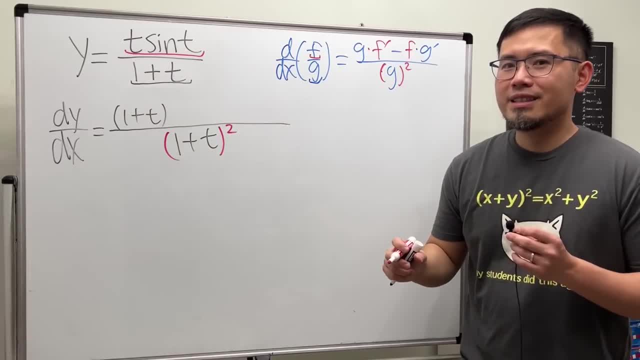 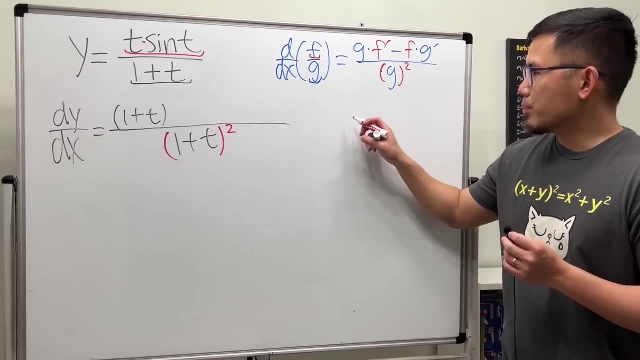 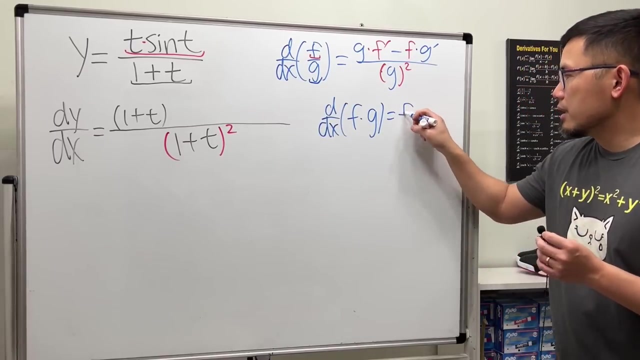 how do we find the derivative of this, The derivative of the top? This right here actually needs a product rule, So let's do it on the side For the product rule. if we differentiate two functions, f times g, this right here is the first function times the derivative of the second. 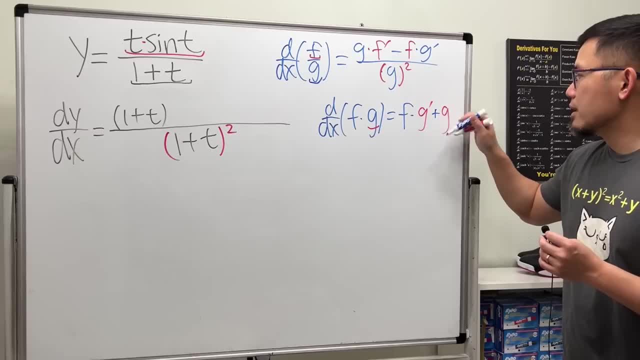 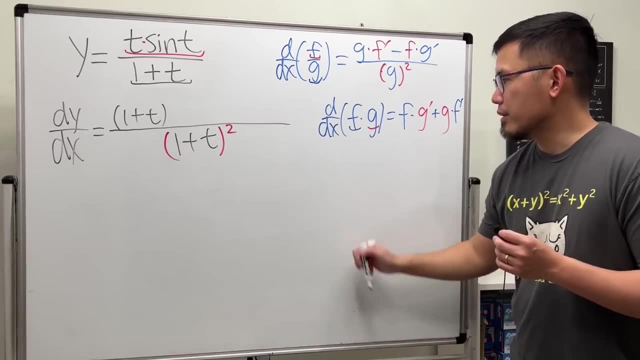 plus the second function times the derivative of the first. And for that- I'm just going to put it down right here- We have to differentiate t times sin t over 1 plus t, and then we have to do it on the other side and we have to do it on the other side. So let's do it on the other side For the product rule. 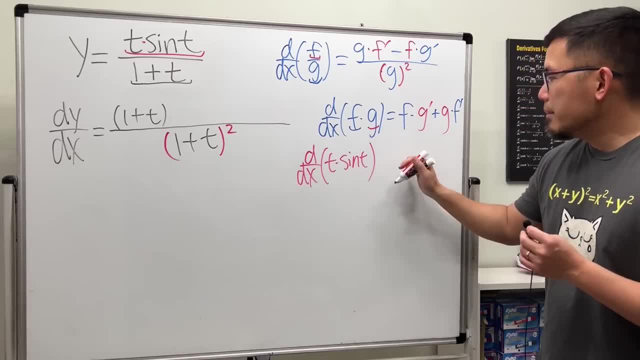 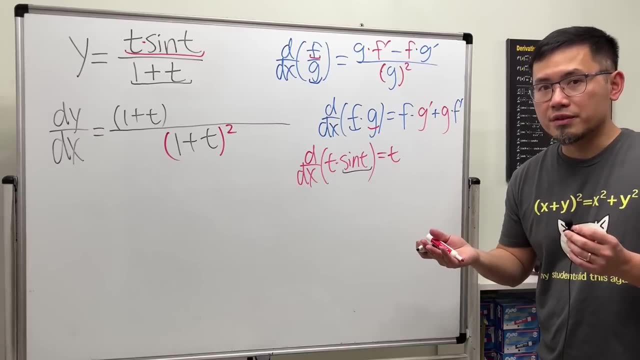 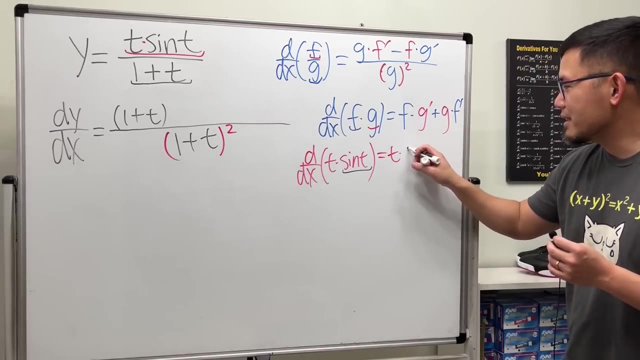 sine T. I'm going to keep the first function, which is just T, and then I'm going to multiply by the derivative of the second, and you have to remember the derivative of sine T, cosine T. yeah, so we have T times cosine T, and then we have: 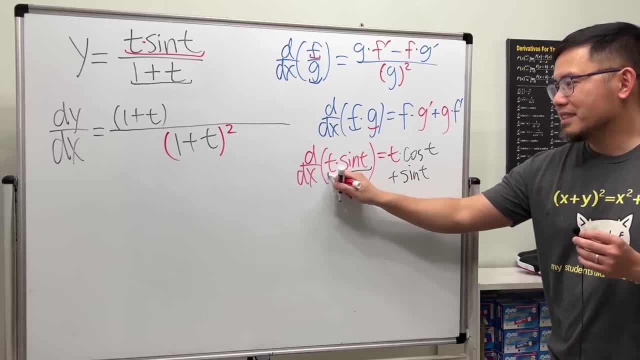 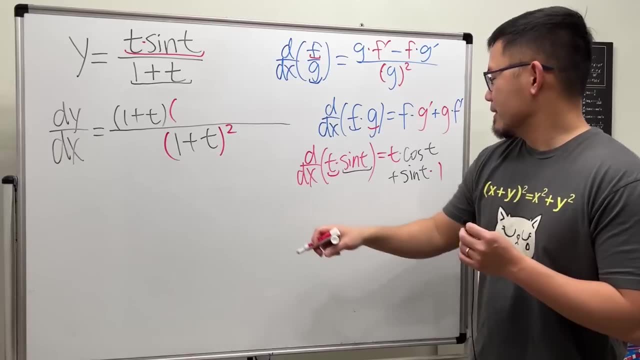 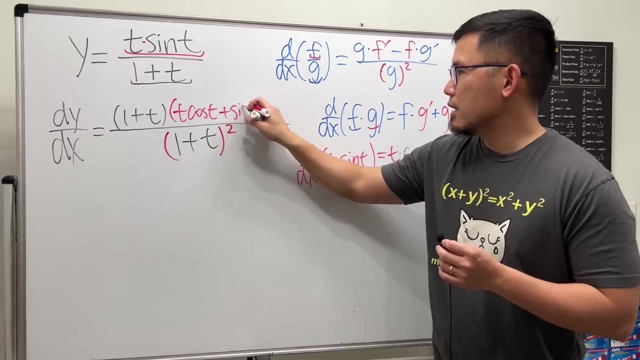 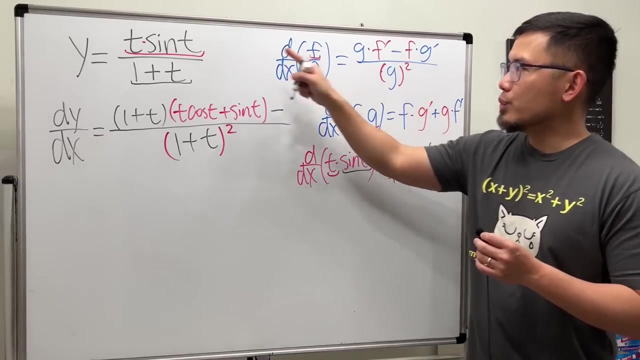 to add a second function, which is sine T times the derivative of the first, which is 1. now put this, multiply with that, so we have T, cosine T and then plus sine T. so that's this part, and then we will have to minus the top function, which is: 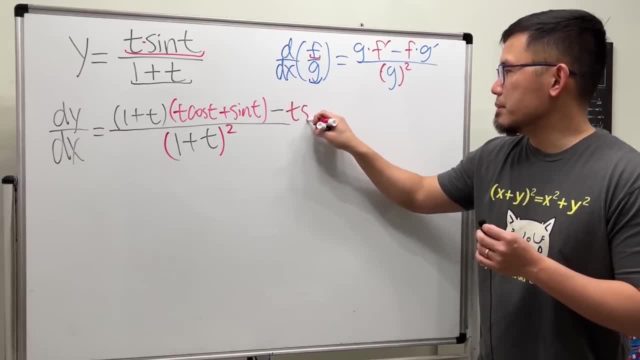 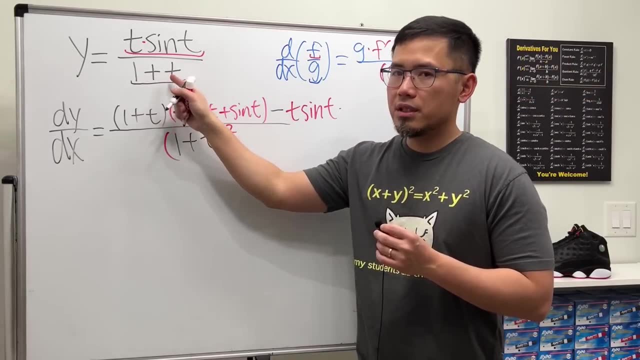 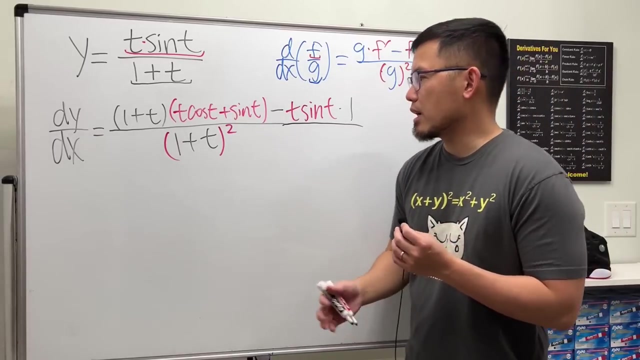 that that is T times sine T. and then we multiply by the derivative of the bottom. the derivative of 1 is 3 wrote. the relative of t is 1. so we multiply by 1. so that's how it looks like then we shall multiply the out and try to see if we can combine any like terms. so on the top i will multiply this. 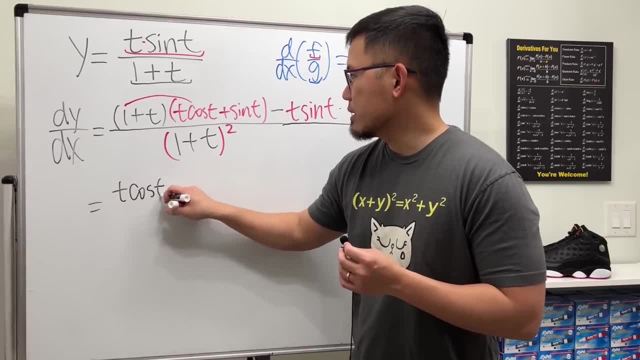 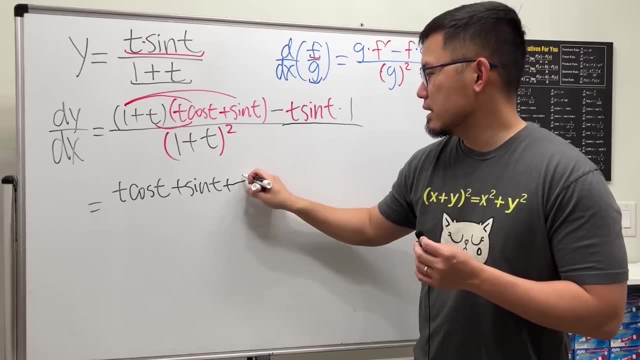 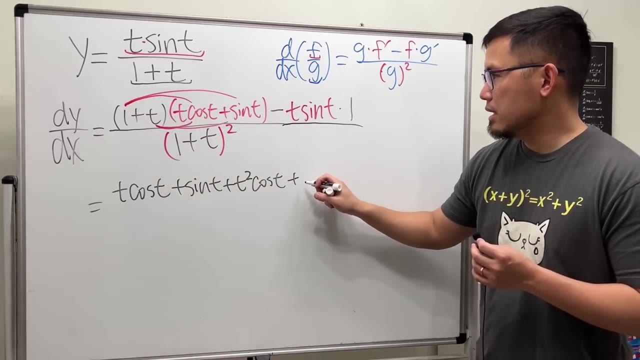 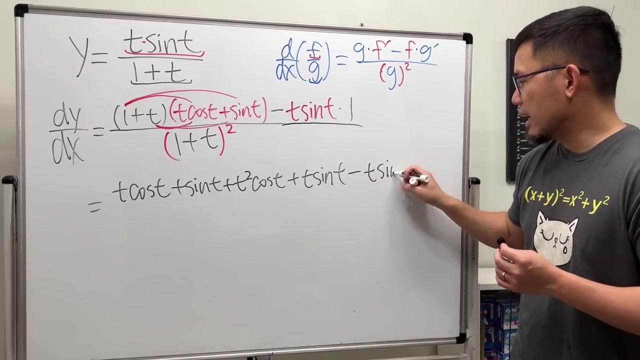 1 times. this is just that. so t cosine t, and then this times that is plus sine t, and then continue with t times that is plus t squared times cosine t, and then, lastly, this times that is plus t sine t. yeah, and then right here we have to minus t sine t, all over that denominator 1 plus t squared. 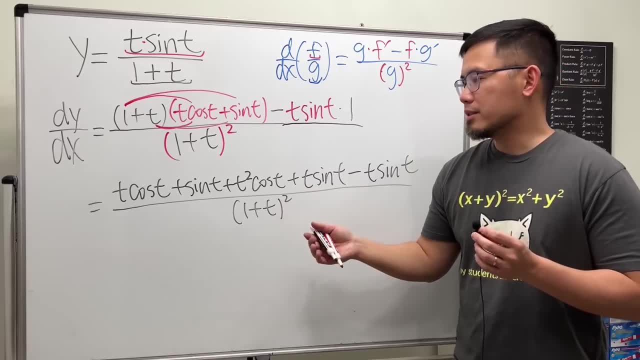 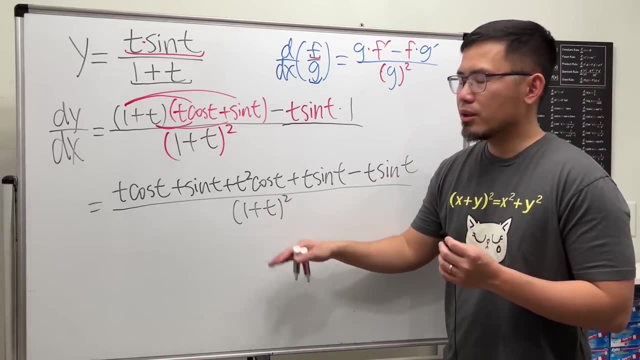 usually you do not have to multiply out the denominator, because the idea is that you want to combine the top and hope that maybe this anything can cancel, so don't multiply it out. and the end. you can really just leave the answer with this right here, if nothing cancels out anyway, though. 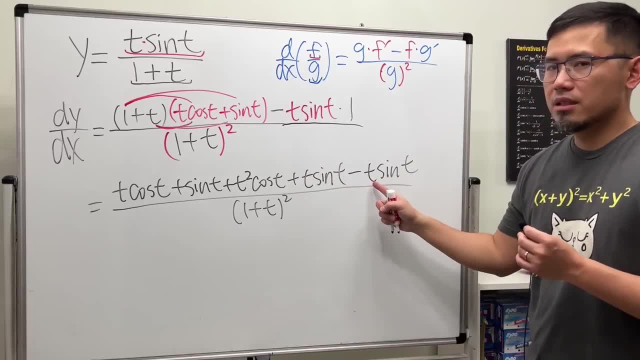 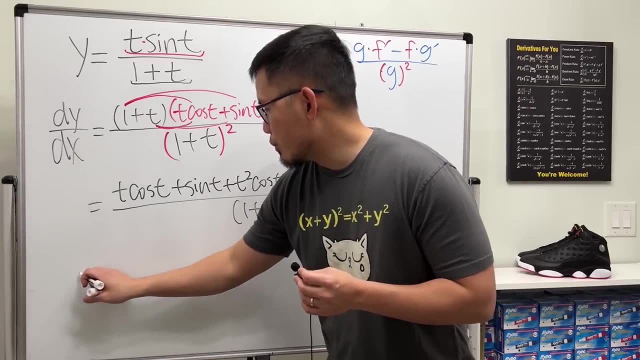 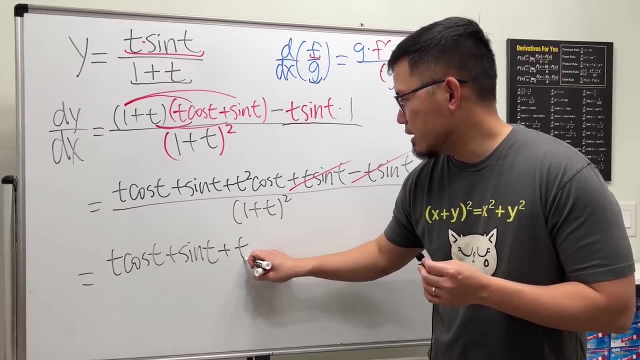 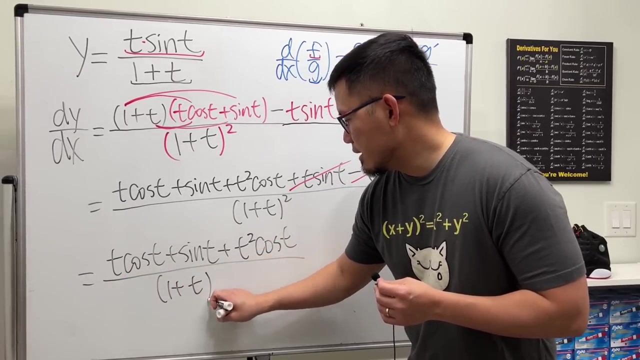 we see that this is positive t sine t and this is a negative t sine t. so bye, bye, and that's pretty much the final answer. i'm just going to write it as t cosine t plus sine t plus t squared, cosine t or over one plus t squared, and that should do it. 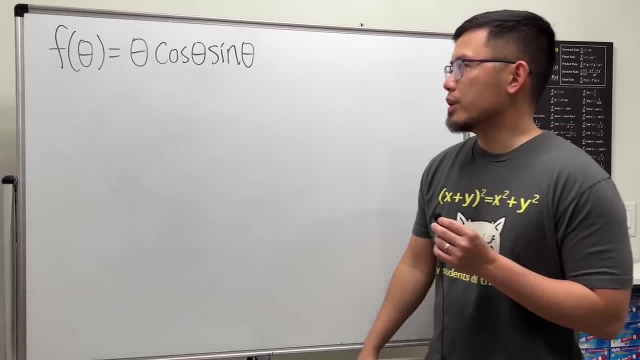 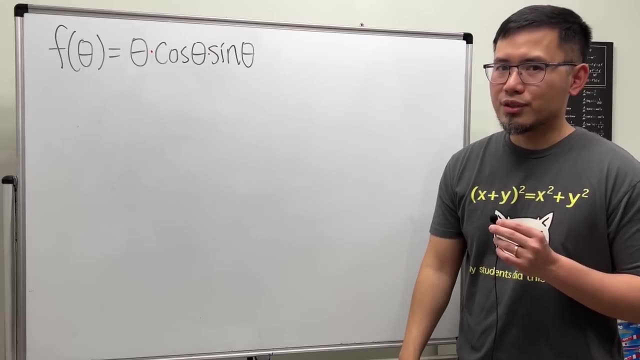 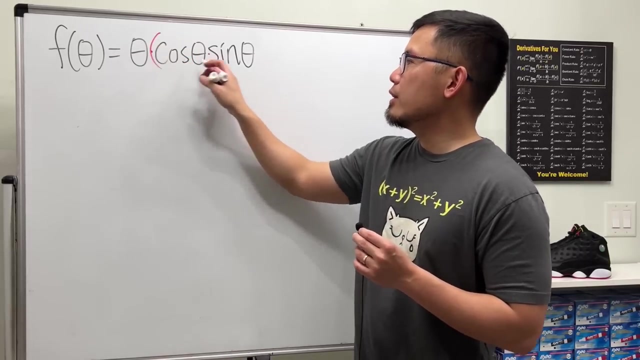 now for the second question. we will differentiate theta times cosine, theta times sine theta. so this is the product of three functions. we still use the product rule, but twice. what we can do is take this as the first function and then group this right here as the second function. right, so i will. 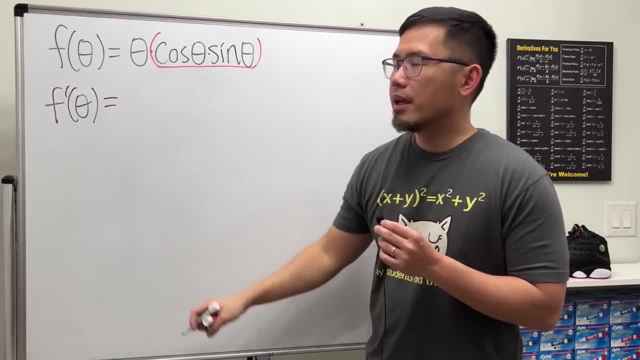 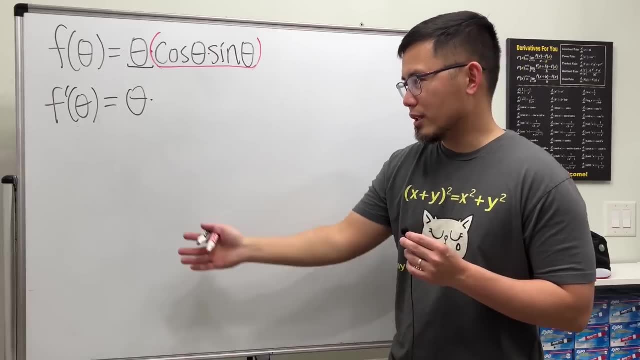 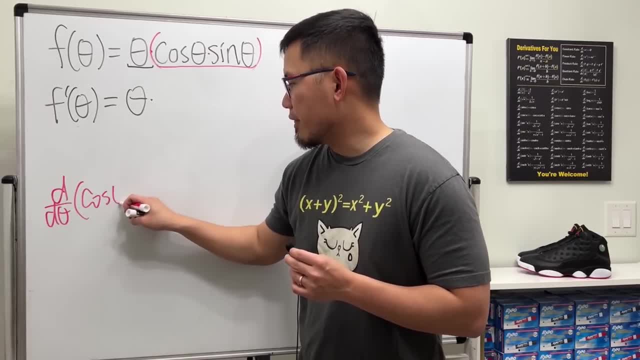 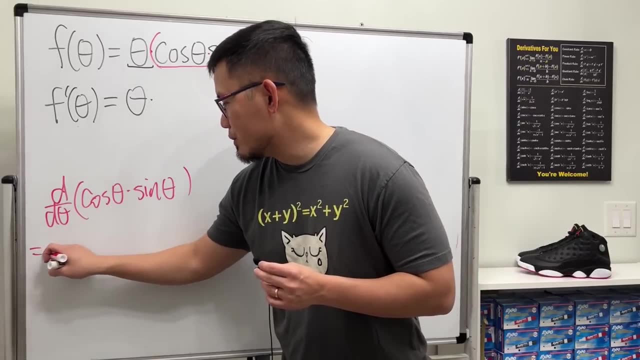 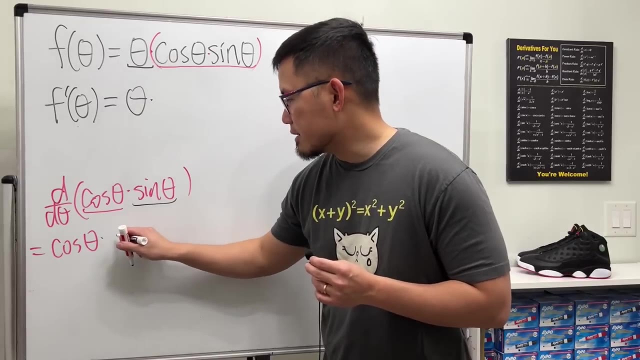 take a look at the derivative of cosine theta times sine theta. of course we need the product rule. i will keep the first function, which is cosine theta, and then i will multiply by the derivative. second derivative of sine theta is cosine theta and then we will have to add the second function. 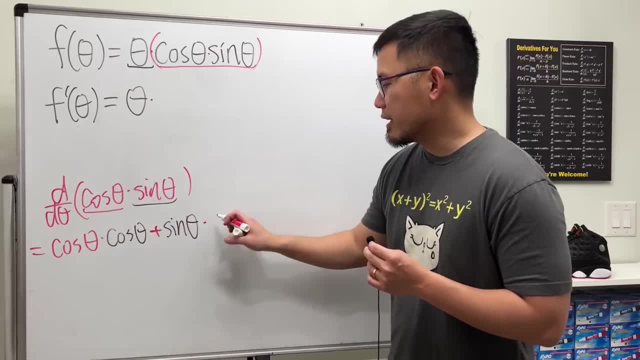 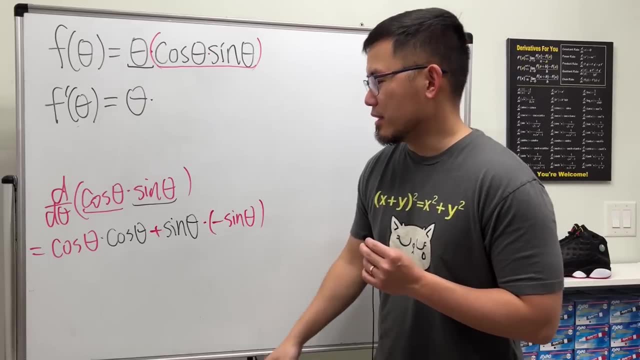 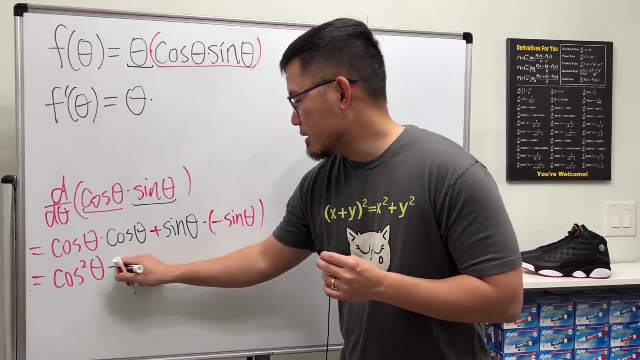 times the derivative of first, the derivative of cosine theta is- we have to remember this carefully- negative sine theta. and we can simplify this a little bit: cosine, cosine is cosine squared, and then theta positive, negative is minus and the sine is the sine which is sine squared theta. here's the deal. 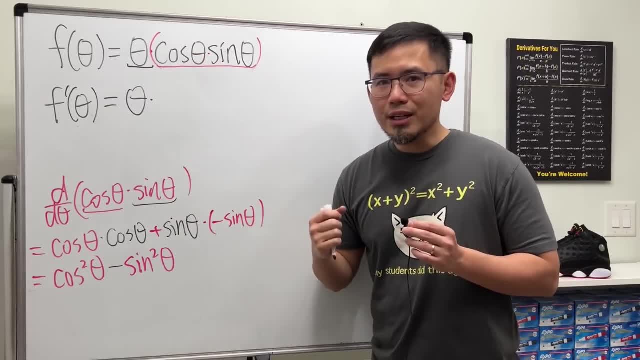 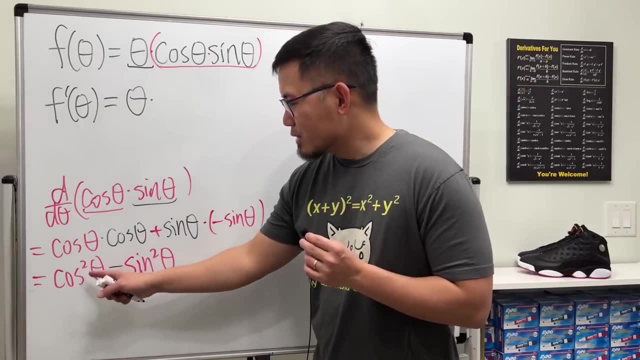 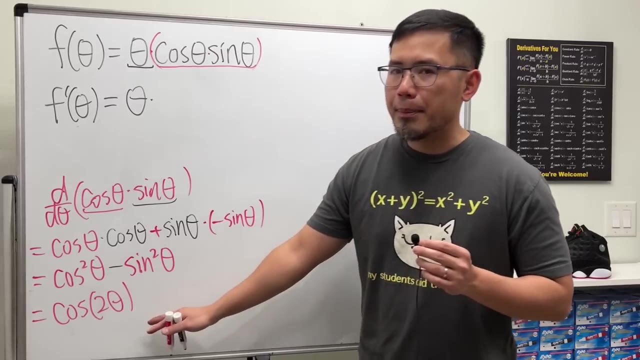 in fact, if you put this down right here for the derivative of this, you're not going to get the answer in the back of the book, because they use the double angle identity to simplify this: cosine squared theta minus sine squared theta. in fact it's the same as cosine of two theta, it's just a double. 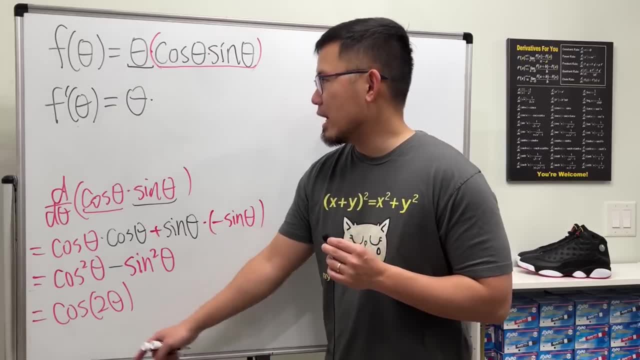 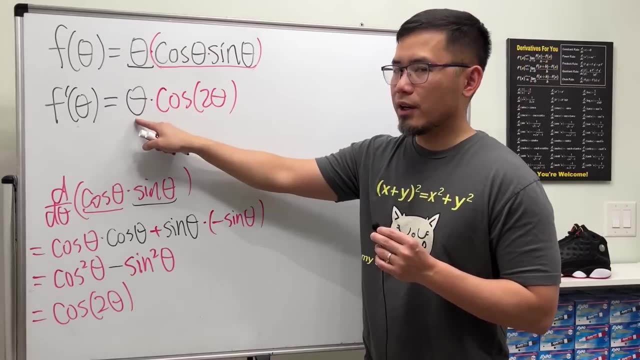 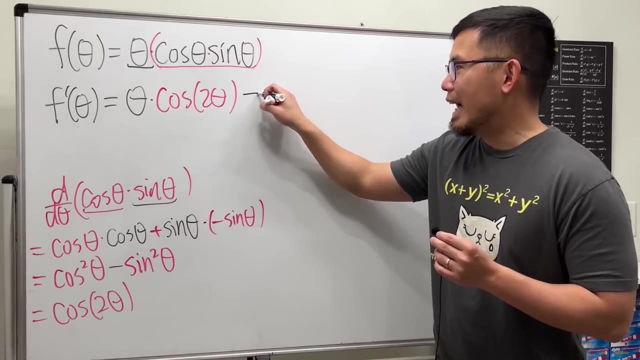 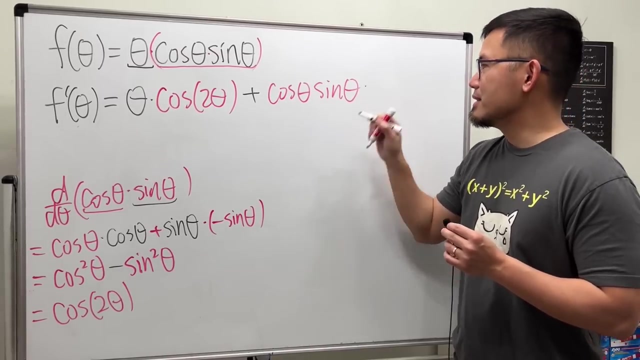 angle identity for cosine. so we will put this down for the derivative of this. so again, we keep the first function times the derivative of the second and the derivative. this is that, and then we have to remember to add the second function, which is that cosine theta sine theta, and then times the derivative of the first. 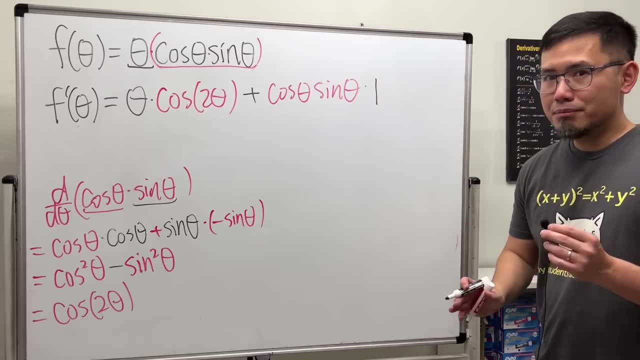 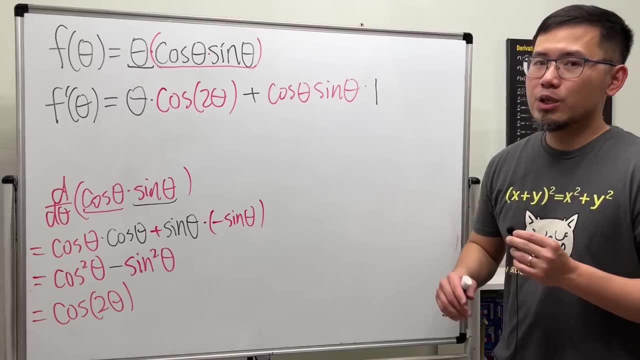 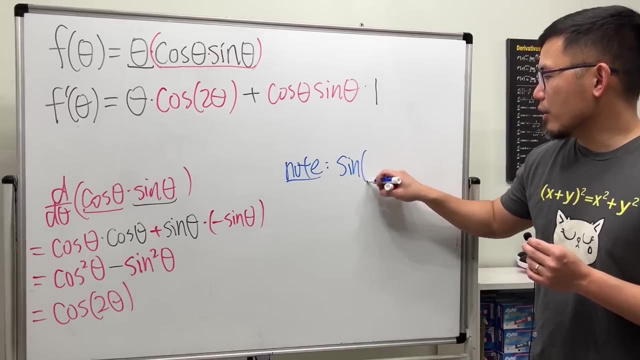 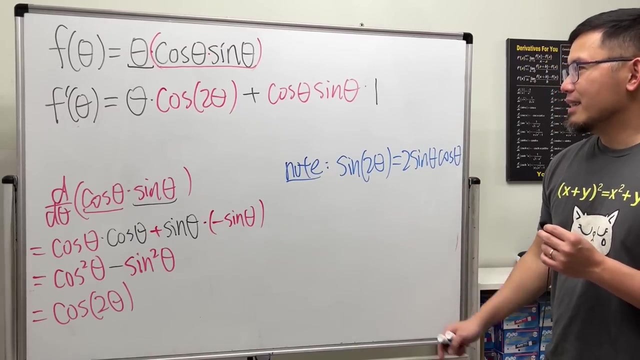 derivative of theta is equal to 1.. are we done almost, because this right here can also be simplified with the double angle identity, but this time it will just be for sine. so let me make a note right here for you real quick. we have sine of two theta. this right here is two sine theta, cosine theta, all right, so of course you. 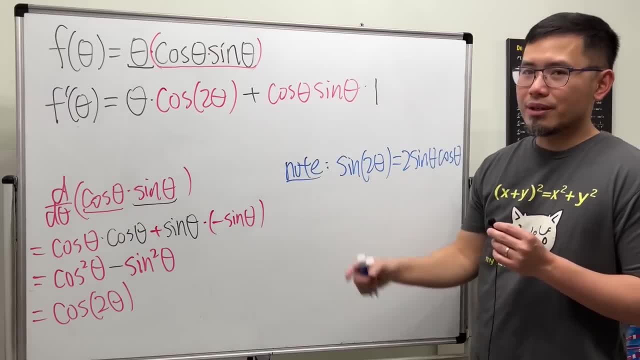 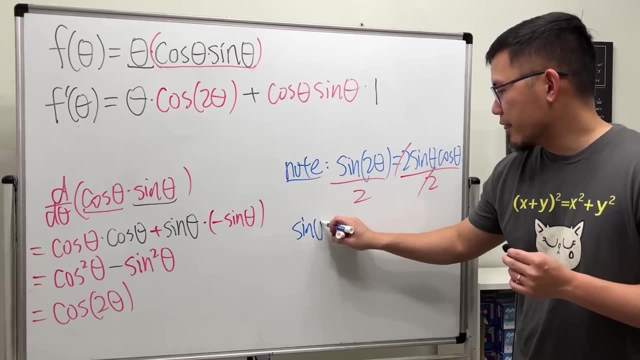 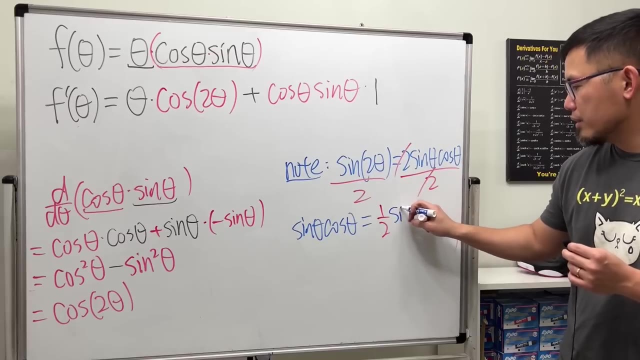 can see that this and that is right here, but we don't have the two here. so just divide both sides by two, so you can see that if we have sine theta times cosine theta, that is just equal to one over two times sine of two theta, and that's exactly what we can put down right here. so at the very